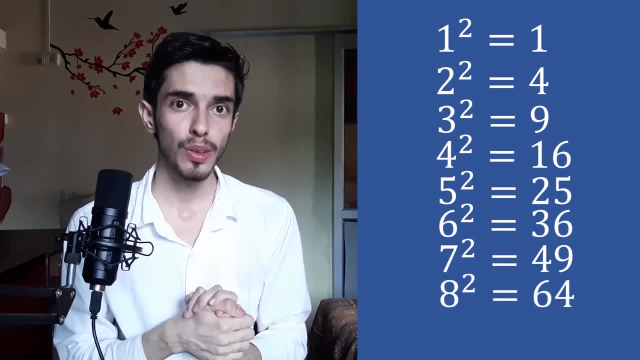 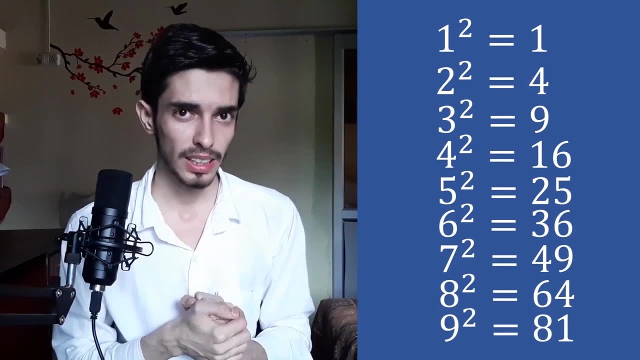 The square of 7 is 49.. The square of 8 is 64.. The square of 9 is 81.. So you need to memorize this by heart before being able to use this trick. And I hope a lot of us already know it, because in our school days we have already learned. 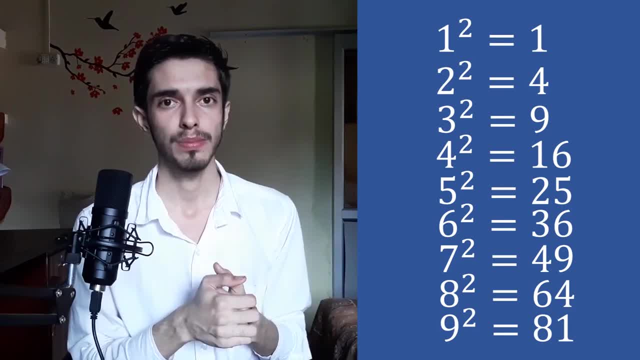 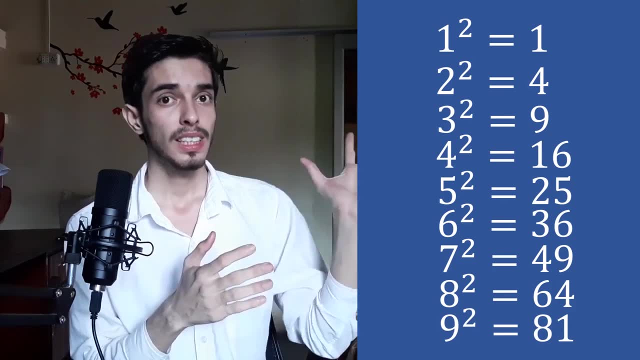 tables from 1 to 10, and we have said it hundreds of times. So most of us should have this thing already memorized, and if you have not memorized this, you should memorize it right now. Now in this, we have a really good pattern in here, which is the key for this trick. The perfect squares ending in 1 will have a root ending in 1 or 9.. The perfect squares ending in 4 will have a root either in 2 or 8.. The perfect squares ending in 9 will have a root either in 3 or 7.. 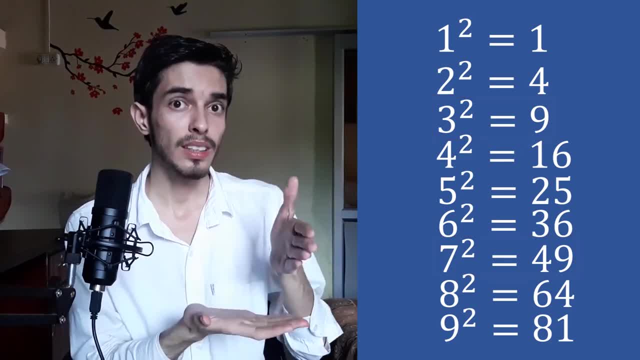 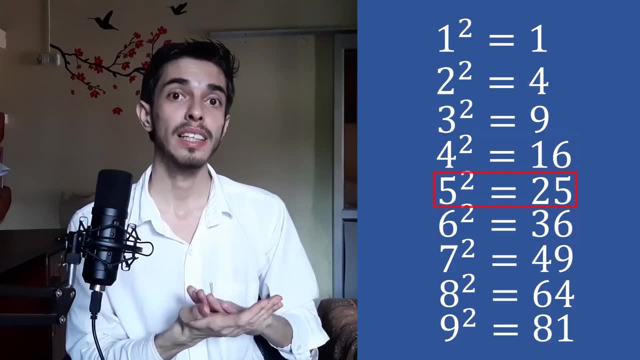 The perfect squares ending in 6 will have a root either in 4 or 6.. And finally, the perfect squares ending in 5 will have a root ending in 5. only Now, with this, let's learn how to find the square root of any 4-digit perfect square. 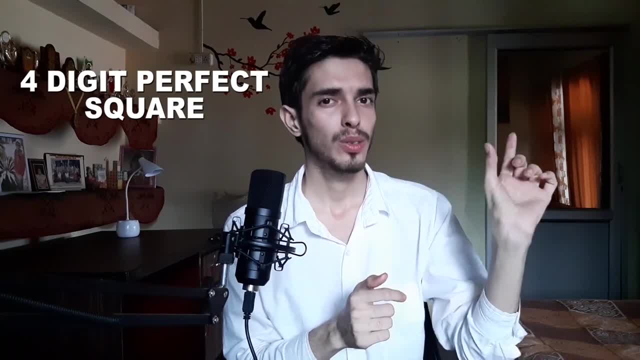 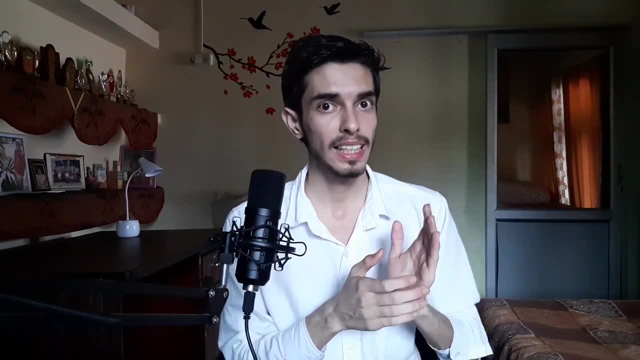 And this is really simple, because a 4-digit perfect square will have a root of 2-digit. Now we have a guess for the last digit of that number, because we know the numbers ending in that would have a root in that. So let's take an example: 6241.. 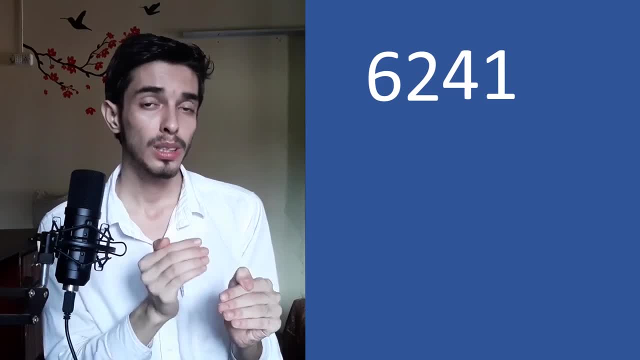 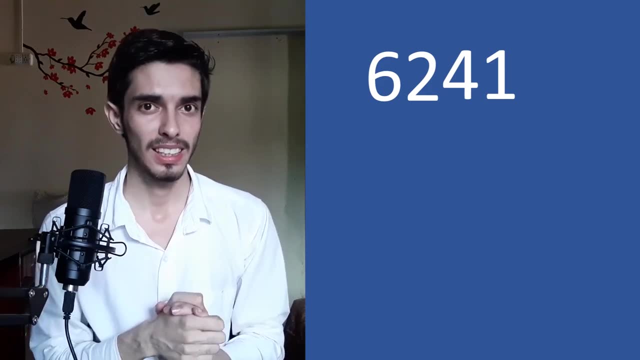 You need to find the square root of this number. Now. first try to do this by yourself, with whatever method you know, And then try the method which I will teach. You will see how good this method is. Now we know that its square root is a 2-digit number. 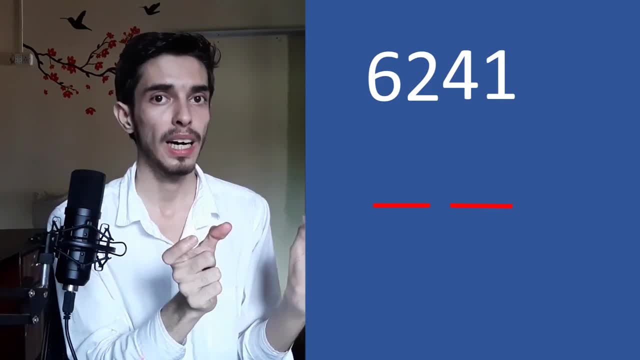 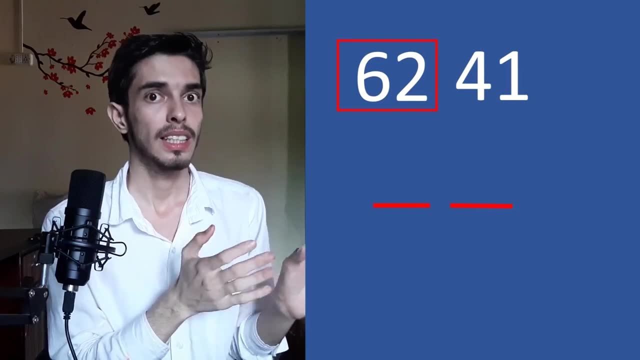 So the first step is to break this number into two parts, which is 62 and 41. Now first focus on this 62.. Seven, sevens are is 49 and eight eights are 64. So 64 is bigger. 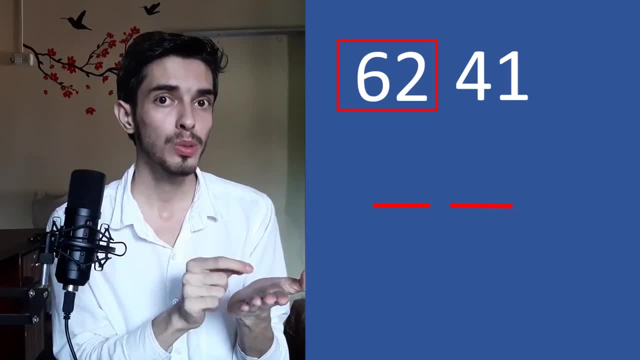 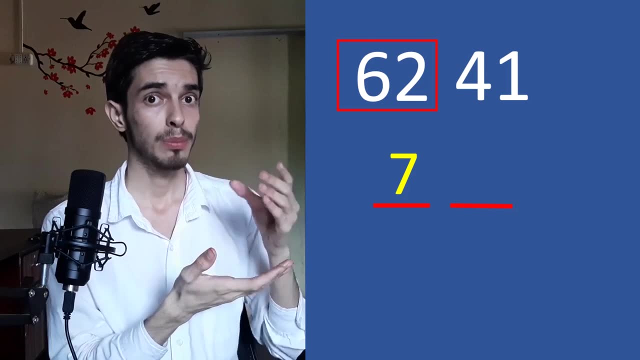 than 62. So the highest possible first digit of the root is 7.. So this is our 1-digit. So from the 2-digits we have the 1-digit. Now step 2 is focus on this. 41. See. 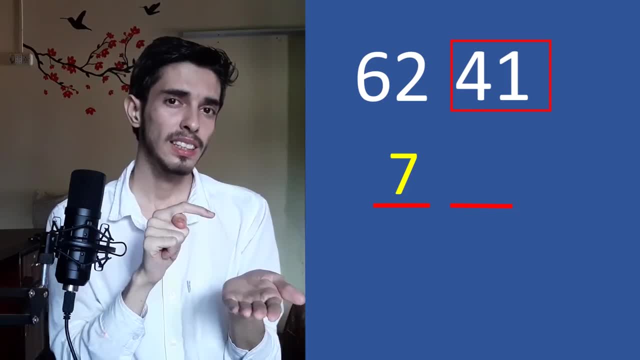 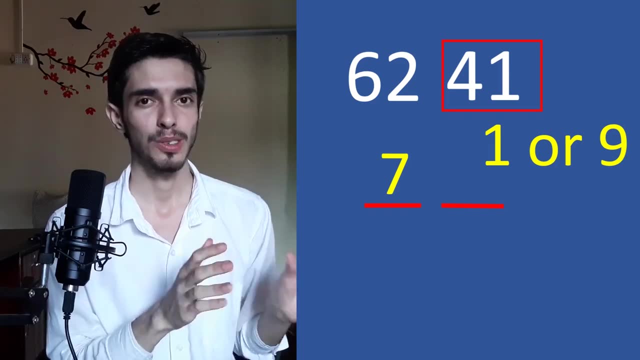 this number is ending in 1.. So the second digit is either 1 or 9.. Now how to choose between these two? This is our task, So this is really simple to do. See, we already know that 7 is the first digit. Now take this digit. 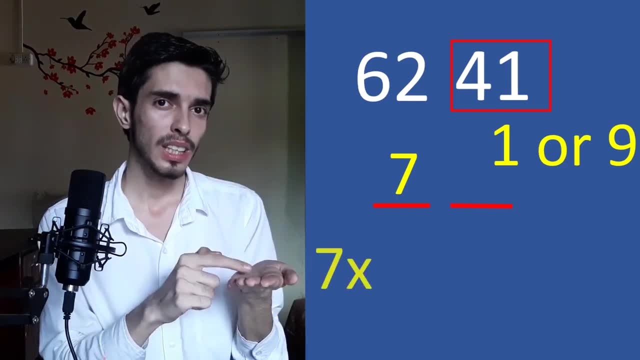 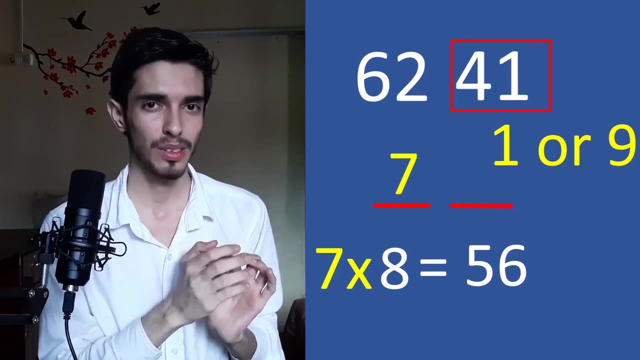 and multiply it with this same digit plus 1.. That is 7 into 7 plus 1., That is 7 into 8.. 8 sevens are 56.. Now here comes a little tricky part, So listen very, very carefully. 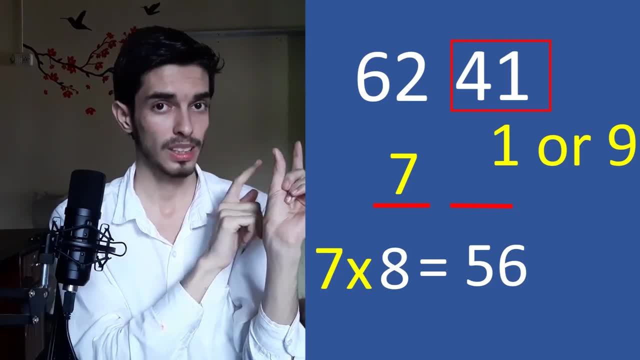 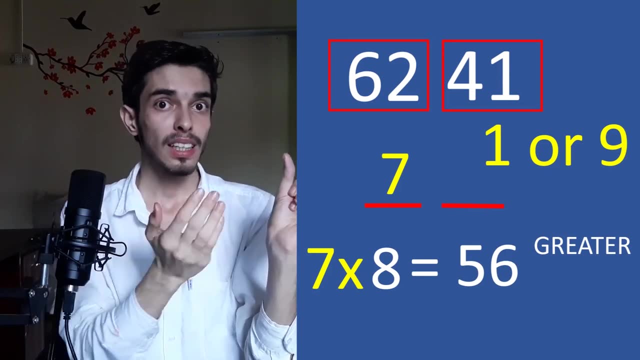 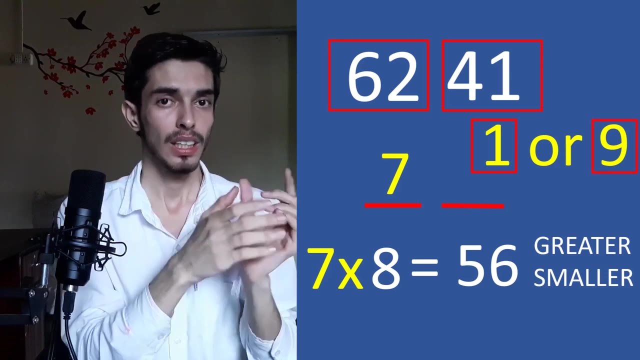 Now, if this number, which is 56 we have got, is greater than the first two digits of our question In here, we have 62. Then take the lower one, which is 1.. And if it is less than those two digits, then take the higher one. So in our case, 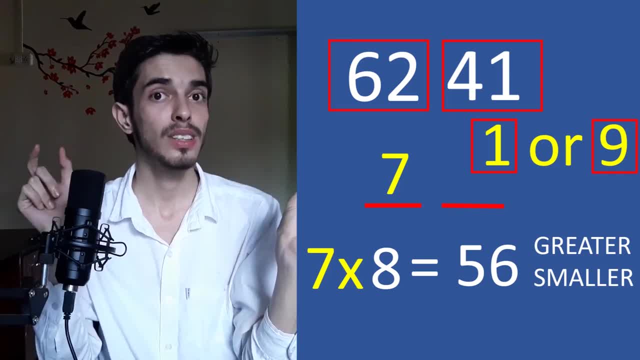 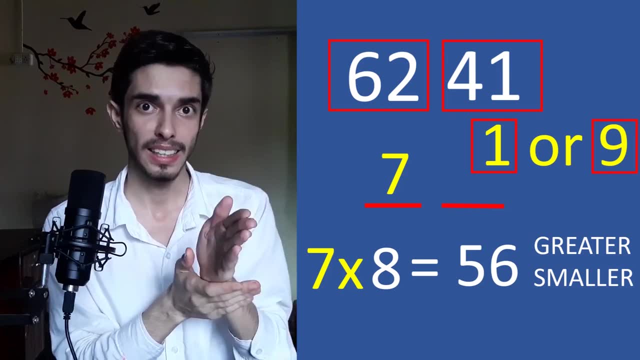 we have 56 and the first two digits are 62. So this is lower one. Then we will go with the higher option, which is we have 1 over 9.. So 9.. So our answer is 79.. So this is how simply we. 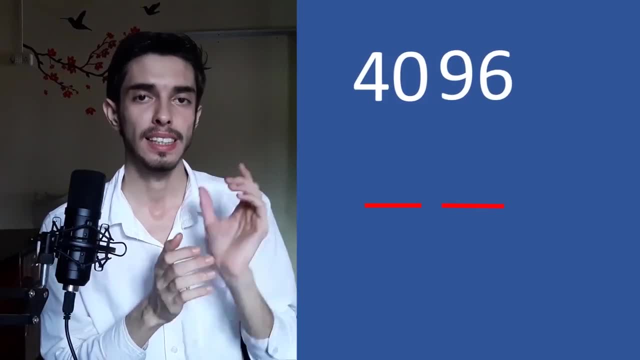 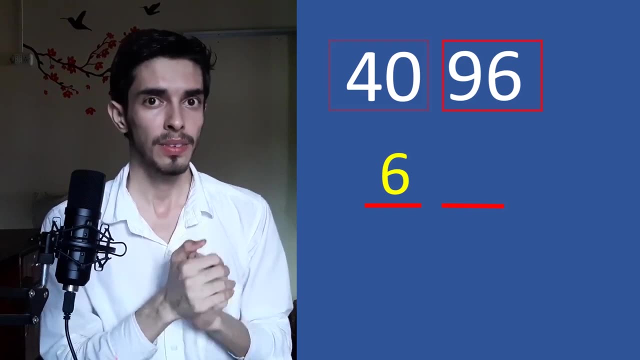 can find square roots. Now let's try another one: 4096.. So 5 halves are 25,, 6, sixths are 36,, 7 sevenths are 49.. So 6 is our first digit. Now this number ends in 6.. So the other number is: 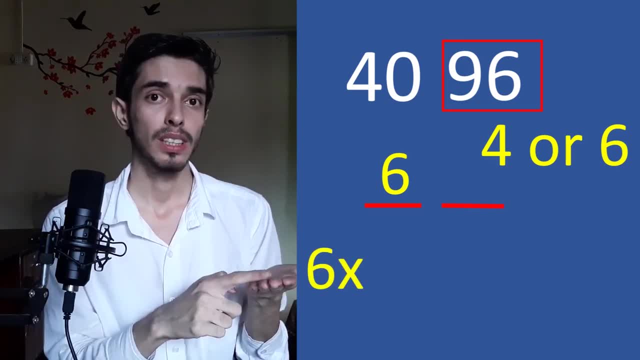 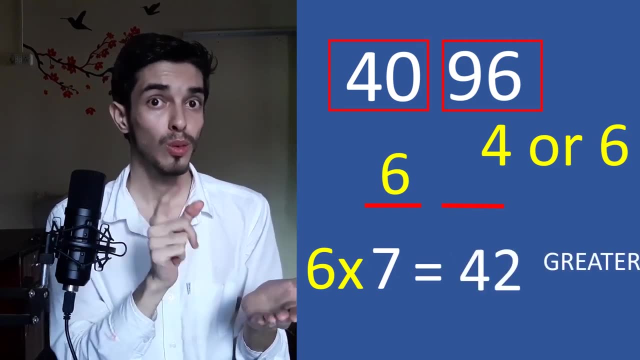 6.. Now which one to choose? So 6 into 6 plus 1.. 6 sevens are 42.. Our first digit is 40.. This is greater, So go with the lower one, 4.. So our answer is 64.. So the square root of 4096 is 64.. 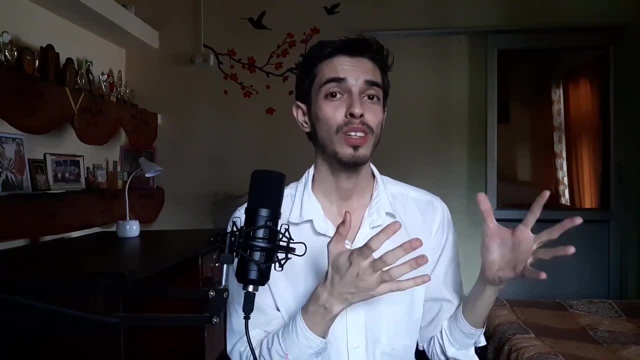 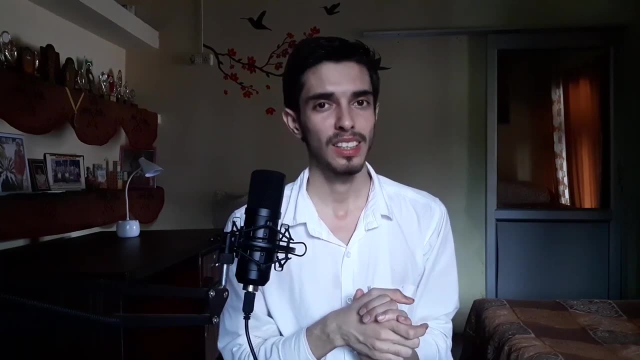 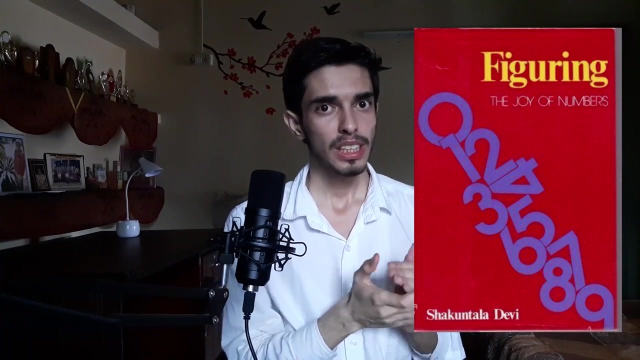 Now this is everything you need to know to find the square root of a 4 digit perfect square, which is amazing Because otherwise your best method was factorization and it would be really long. Now this method which I have taught you is from the book Figuring the Joy of Numbers by Shakuntala Devi. In this book, 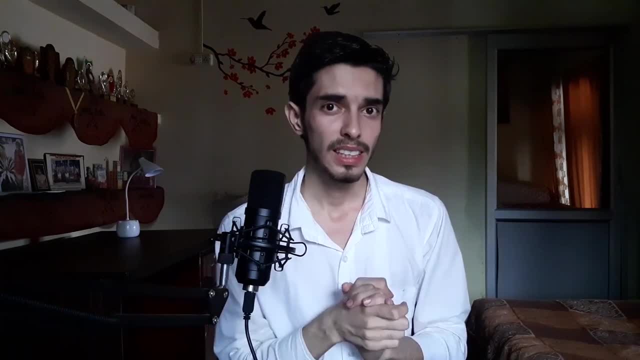 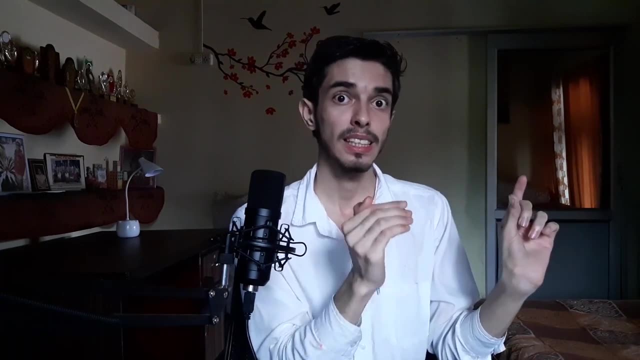 she didn't mention about 3 digit numbers, but I myself figured it out. There is just one exception here: In 4 digit numbers we never had equal to. Like I told you, if that number is greater than that, then go with the lower one, If that number is lower than that, then go with the higher one. But 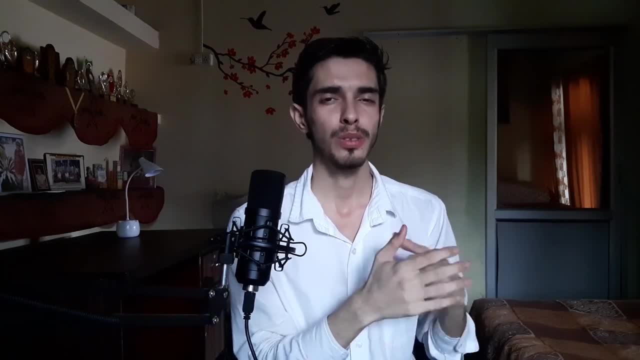 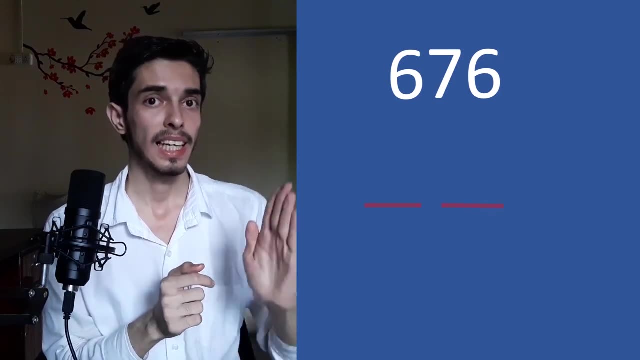 in 3 digit cases we have equal to. Then what do we need to do? So let's learn that with this example. So here is the 3 digit number. So break it like this: 6 and 76.. Now for 6, we have like this, So: 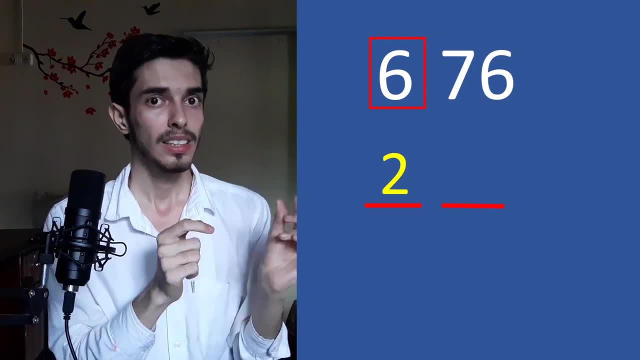 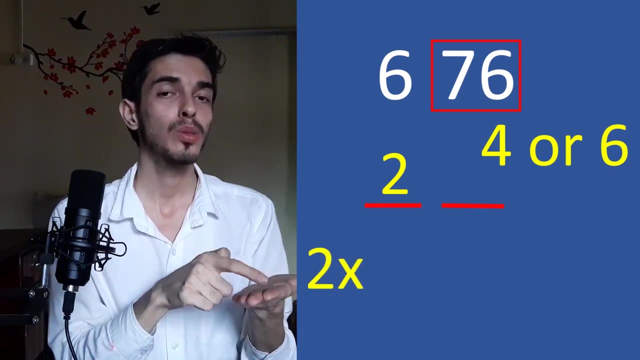 2, 2s are 4 and 3, 3s are 9.. So 2 is our first digit. Now the second digit is either 4 or 6 in here also. So which one to choose? Now 2 into 2 plus 1.. That is two. 3s are 6.. Now the first. 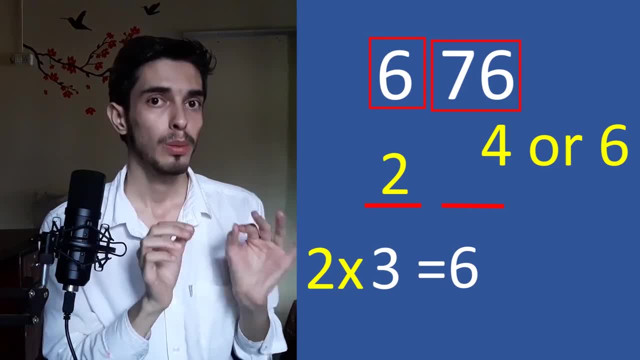 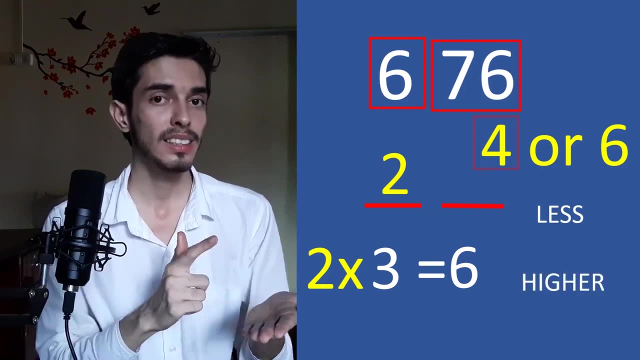 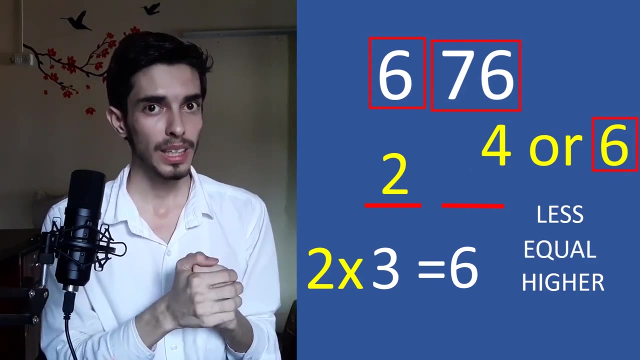 digit is already 6 and we also got 6.. Now, which one to choose? So remember this: If this digit is with the higher one, if this digit is higher than that, then go with the lower one, and if this digit is equal to that, then also go with the higher one. okay, so we had two, and the other one is six. 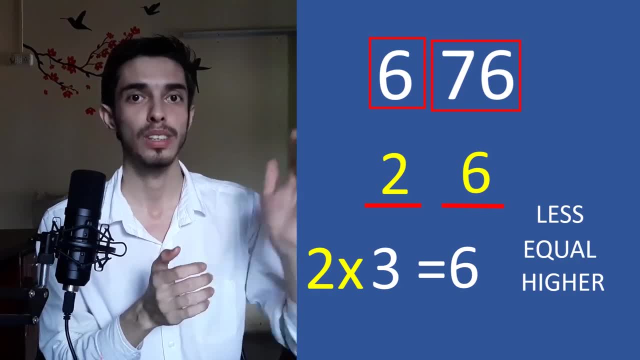 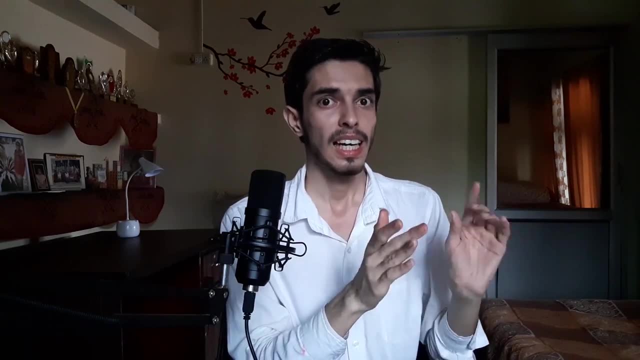 so the answer of this is six, because four is the lower one, so we won't go with that. so this is exactly the same thing you have done with four digit numbers, just in here you split differently and here is equal to case, and in that case go with the higher digit. now let's take 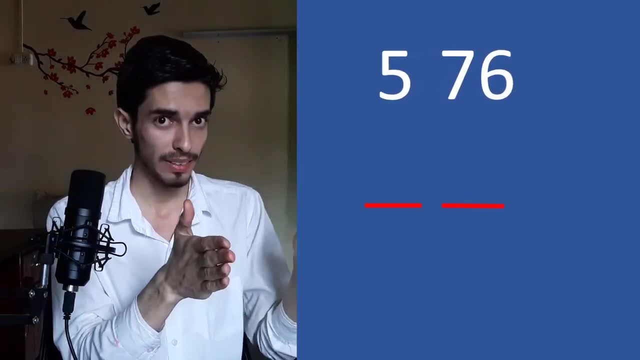 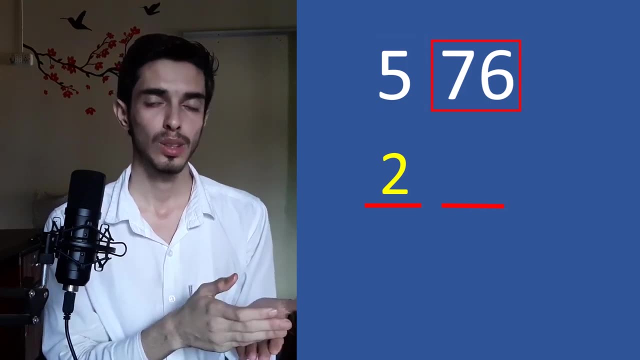 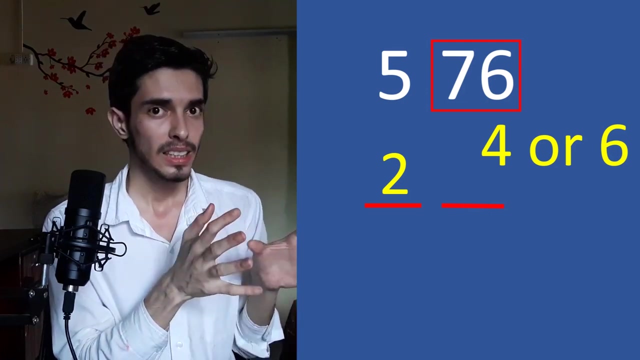 another example: like five, seventy six, so five and seventy six. so one one's a one, two twos are four and three. these are nine, so two and seventy six ends in six. so it is either four or six. you will say why i am taking this same thing like four or six. in previous one it was also four and six. 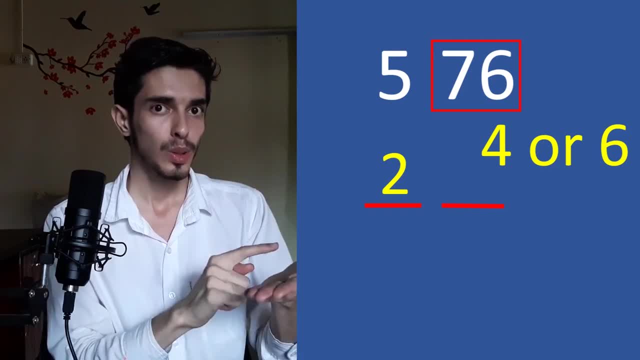 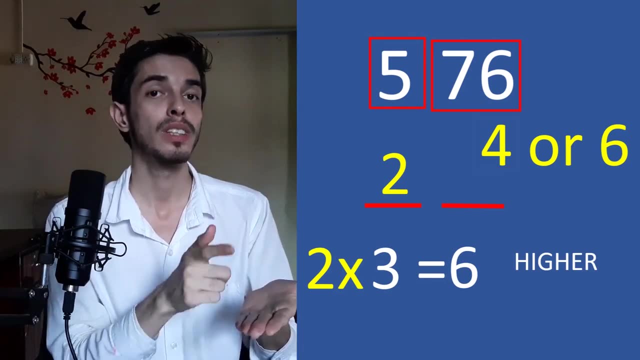 this is just the case in which you will go with four now, because see two into two plus one, which is six. in here our first digit was five, so in here we are higher. so we will go with the lower. so twenty four is the lower one, and we will go with the lower one, so twenty four is the lower one. 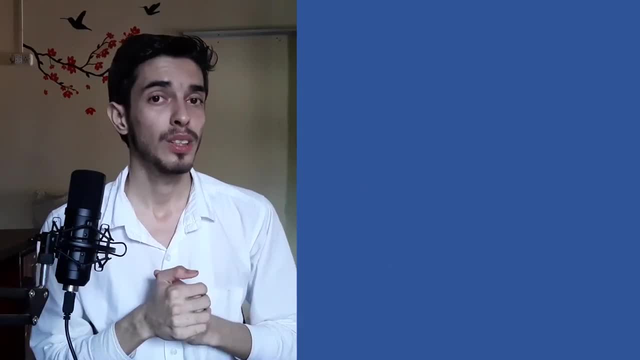 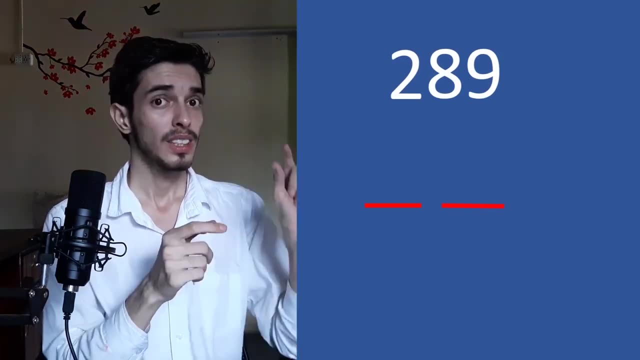 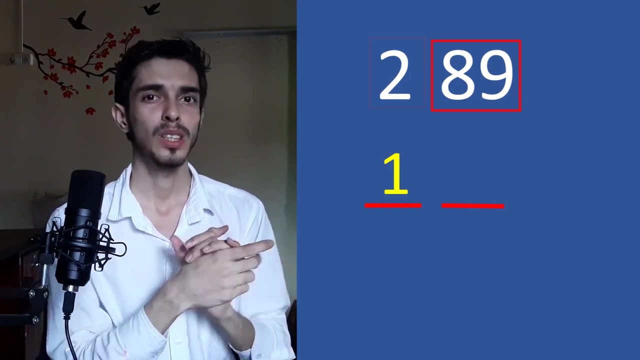 is the square root of 576. so now let's take another, equal to example in three digit numbers: 289. try to do this yourself first. so see two and eighty nine. so one one's a one and two twos are four. so one is our first digit. now let's choose the second digit. this number ends in nine. so what? 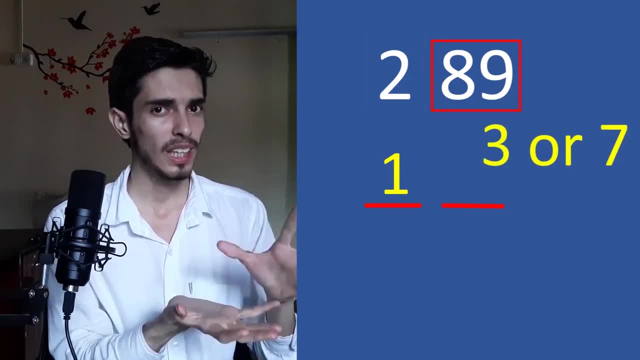 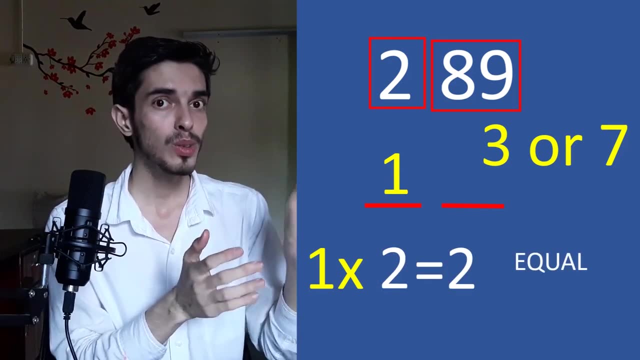 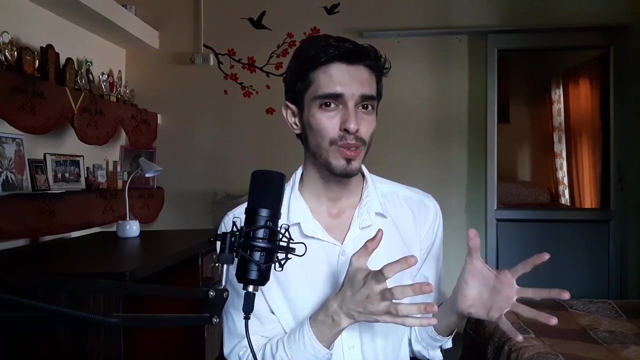 is it? it is either three or seven, so let's choose now one into one plus one, so two and two is equal to this, and whenever this is equal, to go with the greater one, so seven. so our answer is 17.. so this is how we can find square roots of perfect squares of any three digit or four digit numbers. so now,